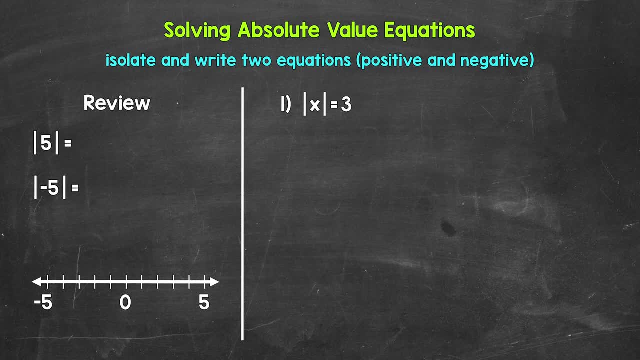 This will give us a solid understanding of absolute value equations. Now, remember the absolute value of a number is its distance from zero. So, for a quick review, the absolute value of five is five. So if we take a look at five on the number line down here, the distance. 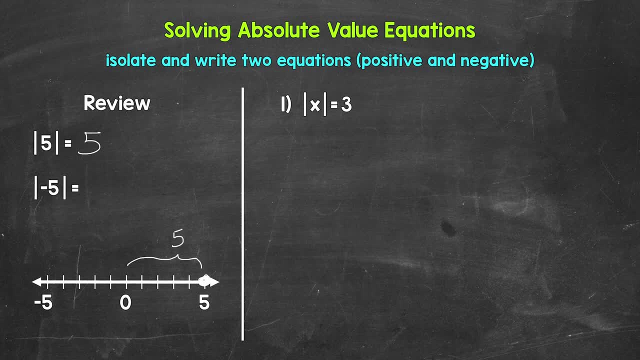 from zero is five units. The absolute value of negative five is five as well And, taking a look at the number line, here's negative five. The distance from zero is also five units for negative five. Keep in mind, the absolute value of a negative is always going to be positive. It's the distance from zero. 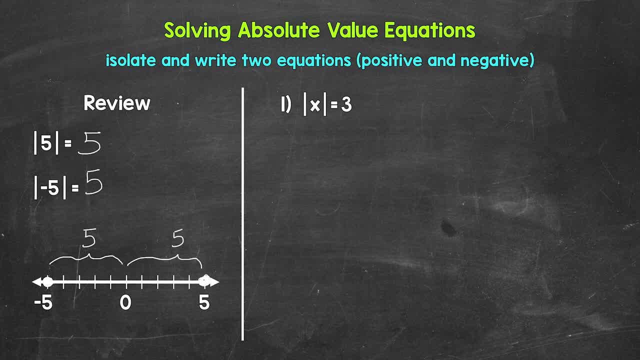 So the absolute value of positive five and negative five is five. Now, going off of this, let's jump into number one, where we have the absolute value of x equals three. Now the first that we want to do is make sure the absolute value is isolated on one side of the equation. 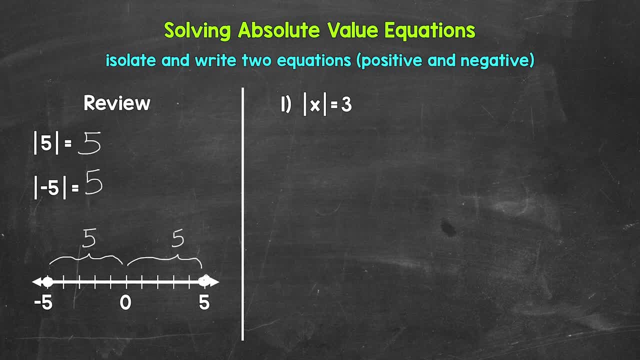 If it's not, we need to start there. For these first three examples, the absolute value will already be isolated. Now, as far as the absolute value of x, it needs to equal three. Well, we have two possibilities here, two solutions. 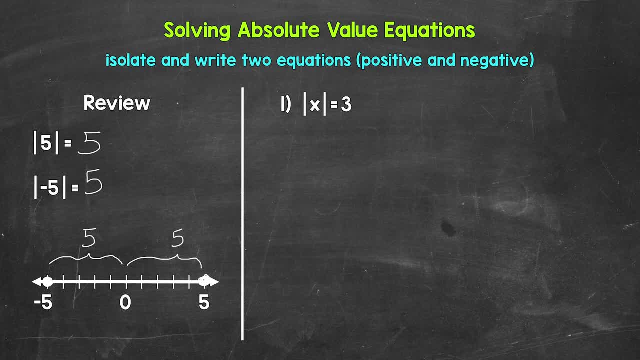 The absolute value of positive three equals three and the absolute value of negative three equals three. Both of those work. So imagine having three or negative three here for x. Both of those are solutions. They both equal three: The absolute value of three. 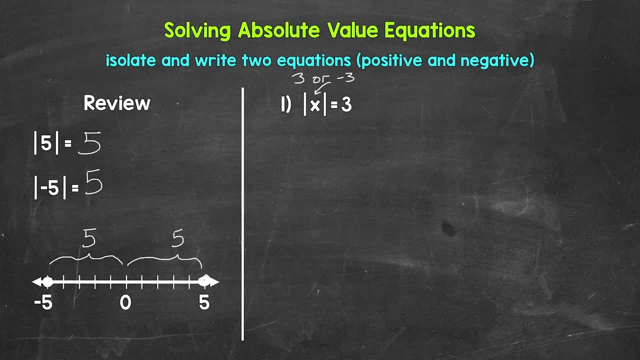 and the absolute value of negative. three equal three. So when we have an absolute value equation, we write two equations: one that is equal to a positive and one that is equal to to a negative. This is going to give us two solutions. Now there are situations where we 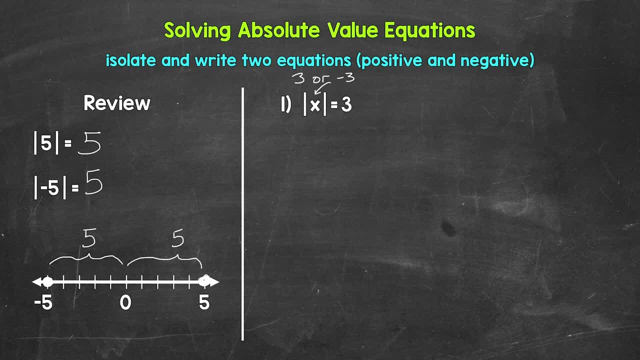 will get one solution or no solution. I'll cover those in another video after this intro. So for number one, x equals three or x equals negative three. Now we can always check our solutions by plugging them in for the variable. So for example, let's come to the side. here We have the absolute. 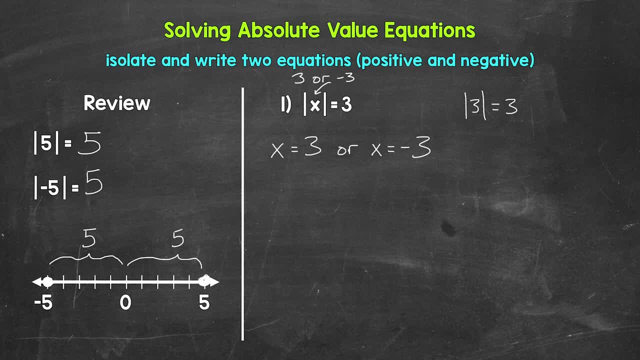 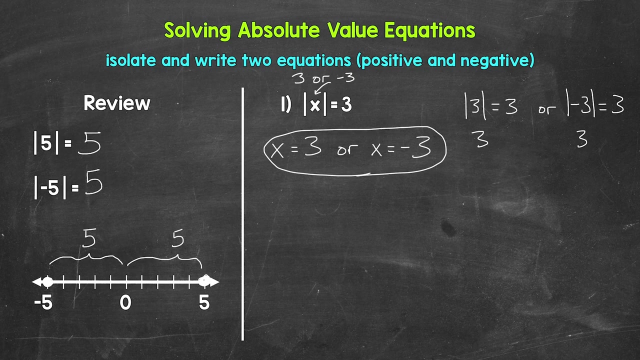 value of three equals three, or the absolute value of negative three equals three. Well, the absolute value of three is three, and then the absolute value of negative three is three. So we do have the correct solutions here. Let's move on Number two and build off of this. Taking a look at number two, we have the absolute value of m plus. 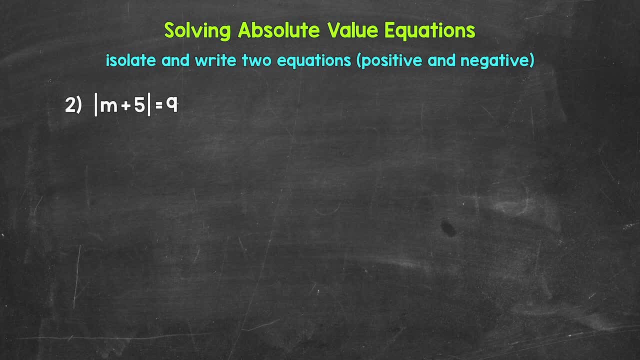 five equals nine. Now our absolute value is isolated here, so we can move on to writing two equations. Now this absolute value equals nine. So we know that m plus five needs to equal positive nine or negative 9.. The absolute value of 9 or negative 9 equals 9.. So we need two equations here: m plus 5. 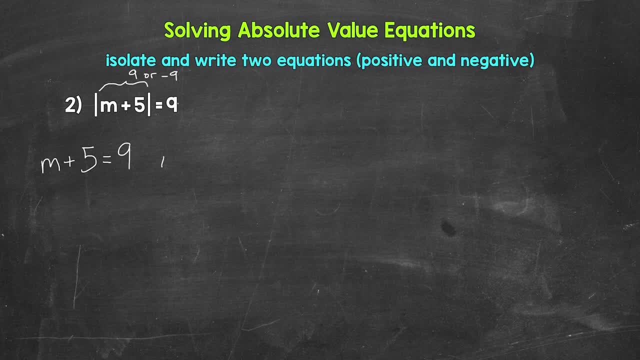 equals 9, or m plus 5 equals negative 9.. Now we solve: Let's start with m plus 5 equals 9.. So we need to isolate that variable of m. We are adding 5 to m, so we need to undo that, The inverse. 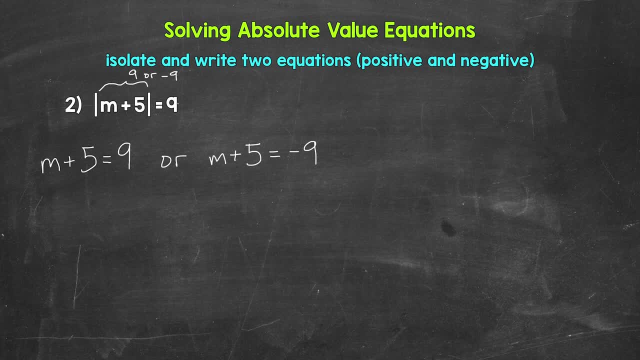 operation of addition is subtraction, So let's subtract 5 from the left side of the equation. Whatever we do to one side, we must do to the other. So subtract 5 from the right side as well. Now, on the left side, we are adding 5 and subtracting 5.. So these 5s cancel each other out. 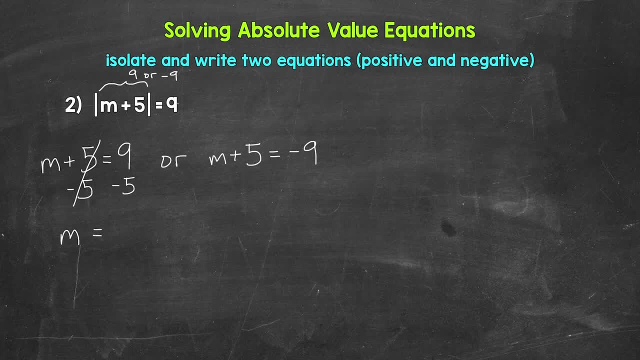 m is now isolated, So m equals. and then on the right side, 9 minus 5 gives us 4.. So m equals 4.. Or let's solve: m plus 5 equals negative 9 now. So we need to isolate m. 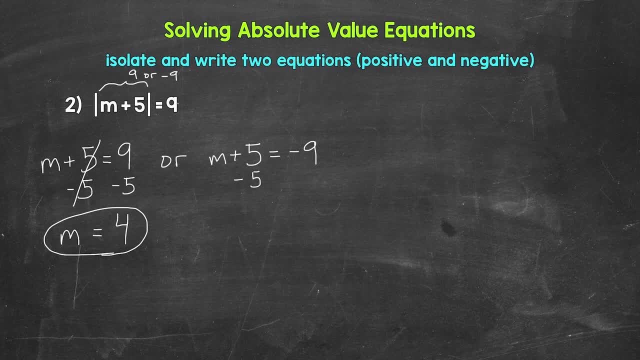 Let's subtract 5 from the left side, That means we need to subtract 5 from the right side as well. These 5s cancel each other out. m is now isolated, So we have m equals. and then on the right side, negative 9 minus 5 gives us negative 14.. So m equals negative. 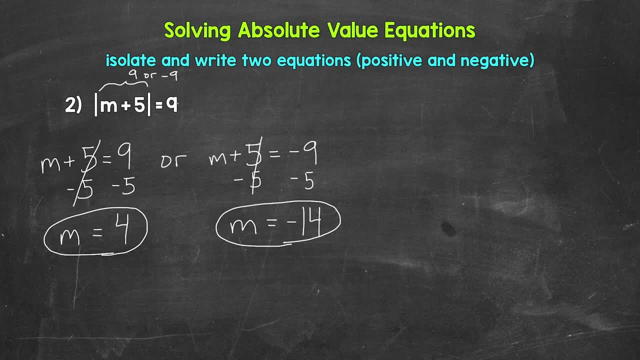 14.. And those are our two solutions. Let's check these solutions by plugging them in for m. So we will start with the absolute value of 4 plus 5 equals 9.. And then we have the absolute value of negative 14.. 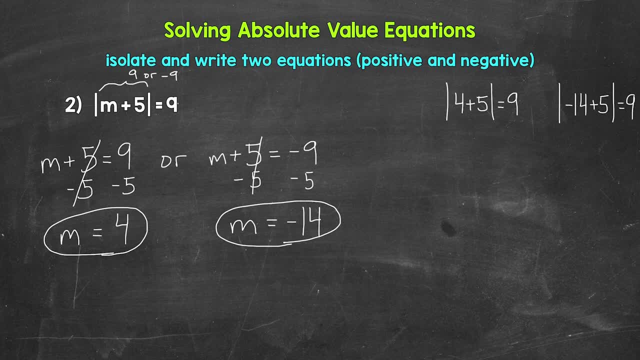 m plus 5 equals 9.. Let's start with the absolute value of 4 plus 5.. Well, 4 plus 5 gives us 9. And the absolute value of 9 is 9.. So that is correct. And then, as far as negative, 14 plus 5,, that gives: 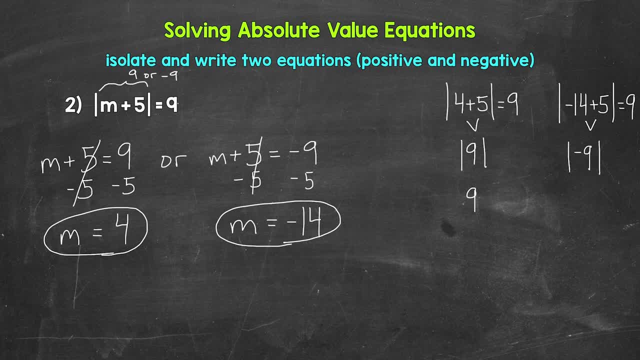 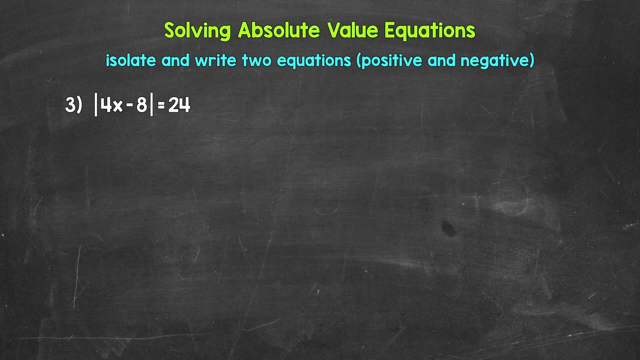 us negative 9.. So we have the absolute value of negative 9.. And that gives us 9 as well. So we are correct, And those are our two solutions. Lastly, let's move on to number 3.. For number 3, we have the. 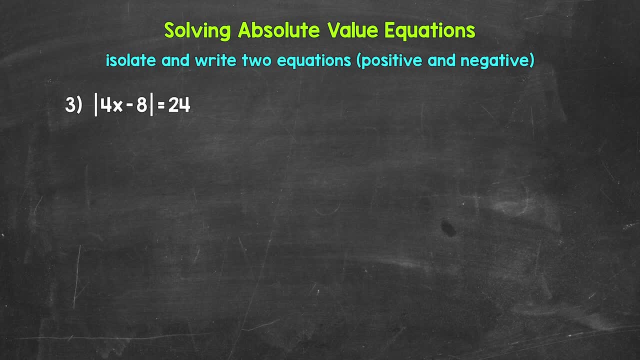 absolute value of 4x minus 8 equals 24.. Our absolute value is isolated, So now we need to write our two equations. So again we have the absolute value of 4x minus 8 equals 24.. That tells us that 4x minus 8 needs to. 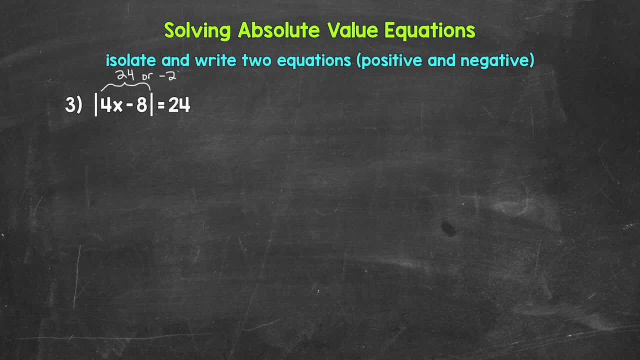 equal 24 or negative 24.. So let's write these equations here: 4x minus 8 equals 24.. Or 4x minus 8 equals negative 24.. And now we can solve. Let's start with 4x minus 8 equals 24.. We need to undo. 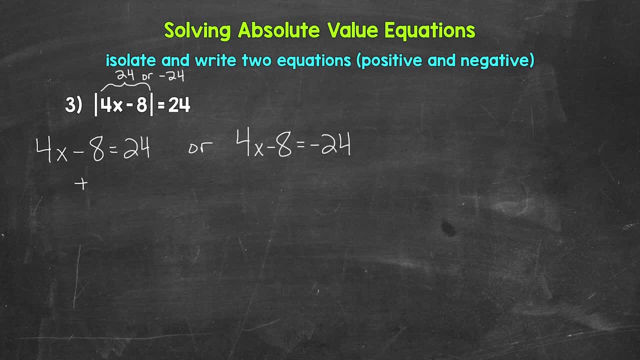 the subtraction, first the inverse operation, And then we have the absolute value of 4x minus 8 equals 24.. So we have the absolute value of 4x minus 8 equals 24.. We need to add 8 to the left. 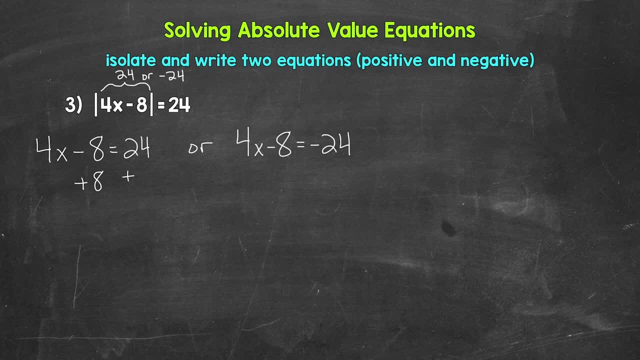 side of the equation, That means we need to add 8 to the right side as well. Now, on the left side of the equation, these 8s cancel each other out, So we have 4x equals. And then on the right side, 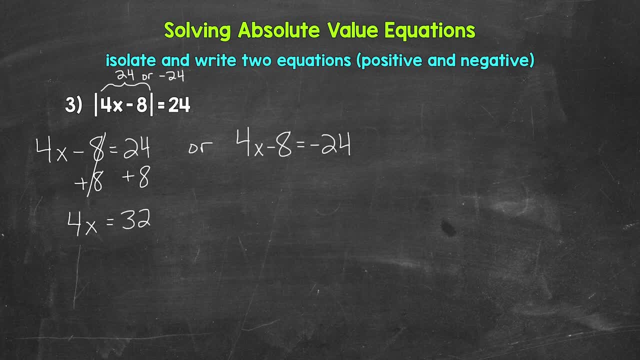 24 plus 8 gives us 32.. Now we have 4x equals 32.. So 4 times x equals 32.. The inverse operation of multiplication is division. So divide the left side by 4.. We need to divide the right side by 4 as well. On the left side these 4s cancel each other out. x is now. 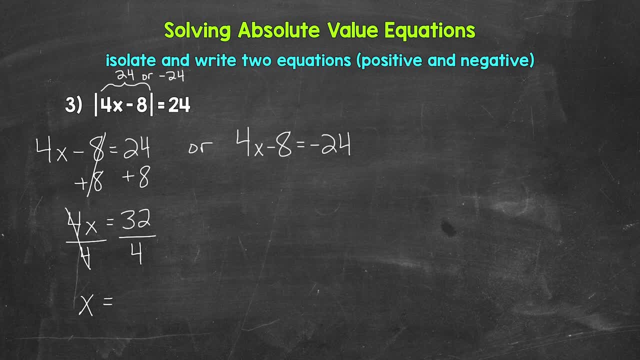 isolated. So we have x equals. And then on the right side, 32 divided by 4 gives us 8.. So x equals 8.. Now let's solve: 4x minus 8 equals 24.. We need to add 8 to the right side of the equation. 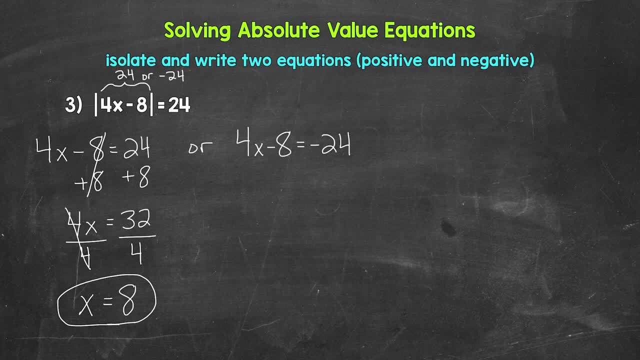 x minus 8 equals negative 24.. So let's add 8 to the left side of the equation and the right side. These cancel each other out. So we have 4x equals. And then on the right, negative 24 plus 8 gives us negative 16.. So let's divide the left side by 4 now. 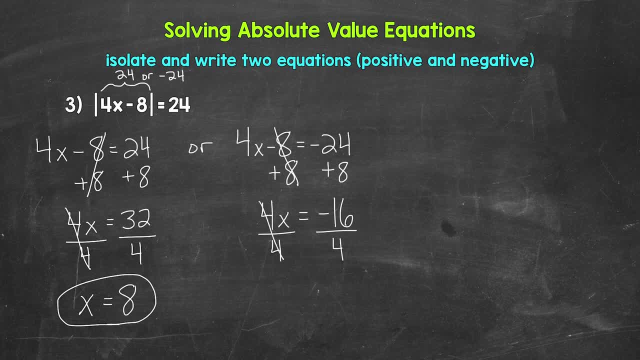 and the right side. These cancel each other out. So we have 4x equals. And then on the right, these 4s cancel each other out. So x is now isolated. We have x equals. And then negative 16 divided by 4 gives us negative 4.. So x equals negative 4.. So those are our two solutions. Let's 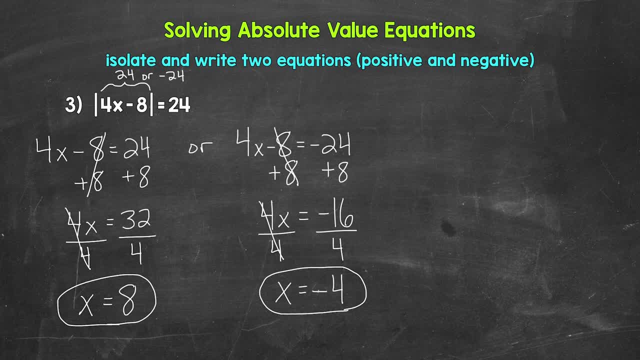 plug those in to see if we are correct. Let's check those. So we have the absolute value of 4 times 8 minus 8.. x equals 24.. And then we also have the absolute value of 4 times negative. 4 minus 8 equals 24.. 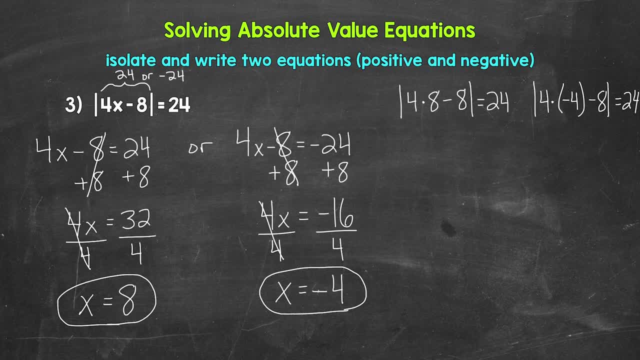 Let's start with the absolute value of 4 times 8 minus 8.. 4 times 8 is 32.. So now we have the absolute value of 32 minus 8.. 32 minus 8 gives us 24.. And the absolute value of 4 times 8 minus 8. 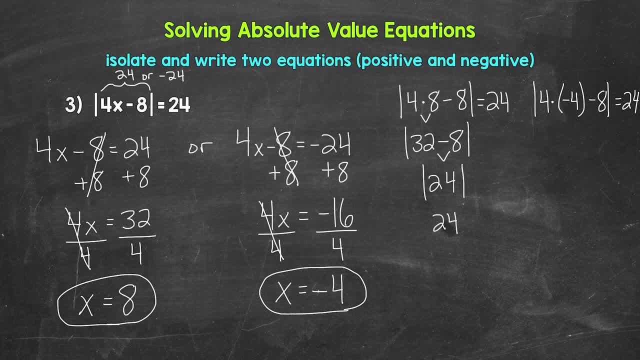 is 24.. So we are correct. there, x equals 8.. Now let's do the absolute value of 4 times negative, 4 minus 8.. 4 times negative, 4 is negative 16. So we have the absolute value of negative 16 minus 8.. 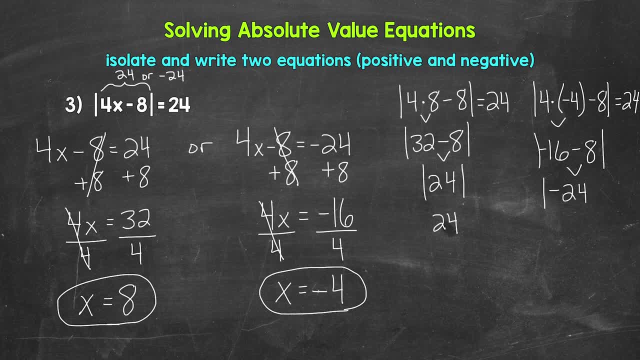 That gives us negative 24.. So we have the absolute value of negative 24,, which is also 24.. So we are correct there as well. x equals negative 4.. So those are our two solutions. So there's our first section. Let's move on to our second section, where we will have numbers and operations outside. 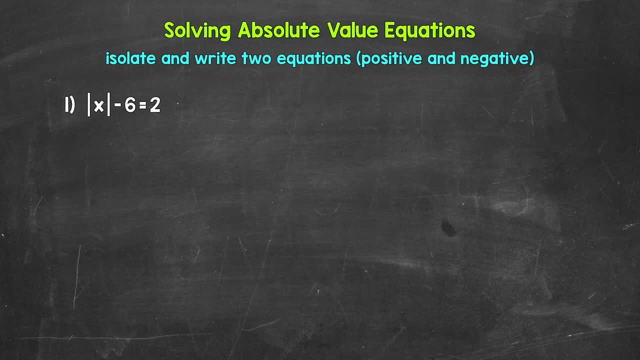 of the absolute value. Here's our second section. Let's jump into number one, where we have the absolute value of x minus 6 equals 2.. Now remember, the first thing that we need to do when we have an absolute value equation is look to see if the absolute 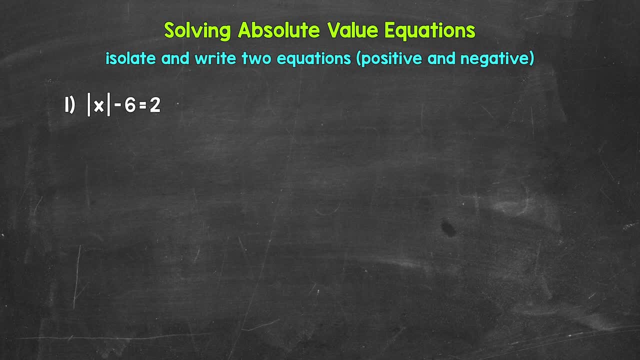 value is isolated on one side of the equation, So it needs to be by itself on one side of the equation. In this example, the absolute value is not isolated. It's not by itself. We are subtracting 6 from it. That means we need to start by isolating the absolute value. We need to undo. 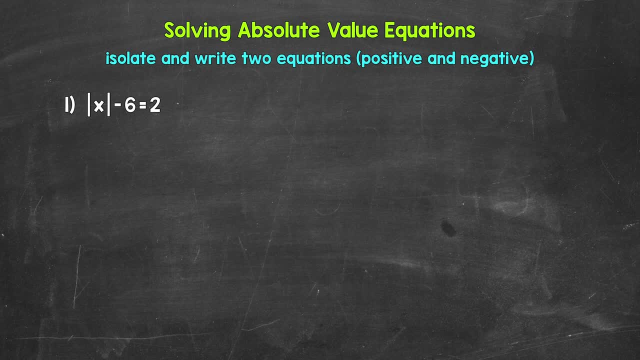 that subtraction, The inverse operation of the absolute value, is not isolated. We need to start. subtraction is addition, So let's add 6 to the left side of the equation. Whatever we do to one side of an equation, we must do to the other, So add 6 to the right side as well. Taking a look at: 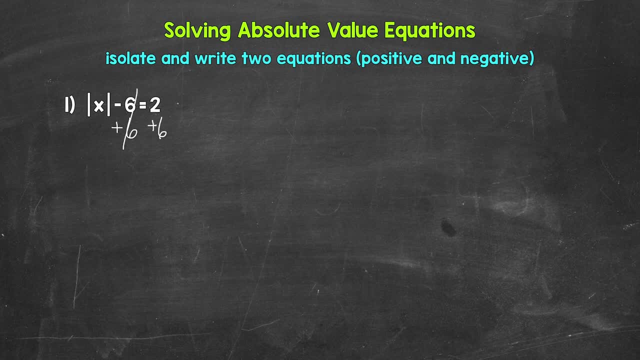 the left side of the equation, these 6s cancel each other out. So now we have the absolute value of x equals, and then, on the right side of the equation, gives us 8.. So now we have the absolute value of x equals 8.. Now, keep in mind, we know that the 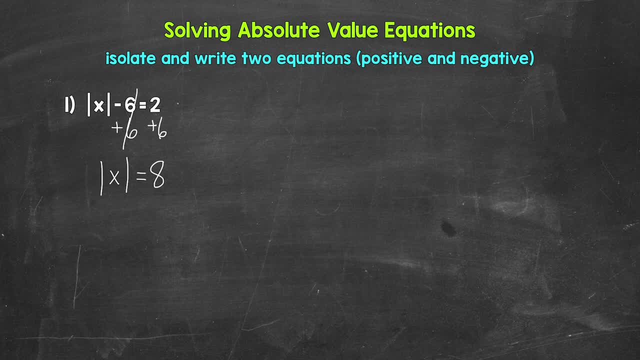 absolute value of positive 8 equals 8, and we know that the absolute value of negative 8 equals 8.. So x can be 8 or negative 8.. So this is where we write two equations. We have two options here. 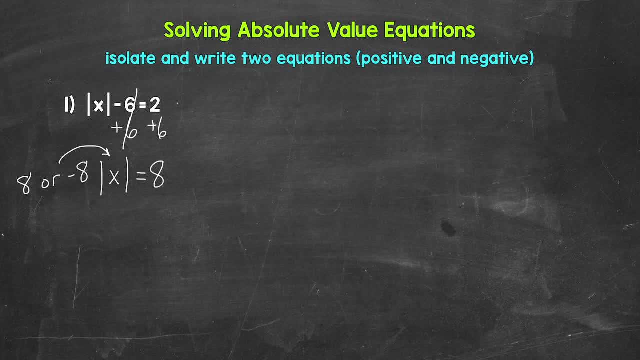 two scenarios. We are going to give us two solutions. So x equals 8 or x equals negative 8.. Now here, for this example, the variable is already isolated. We have x equals 8 or x equals negative 8.. So we are done here. 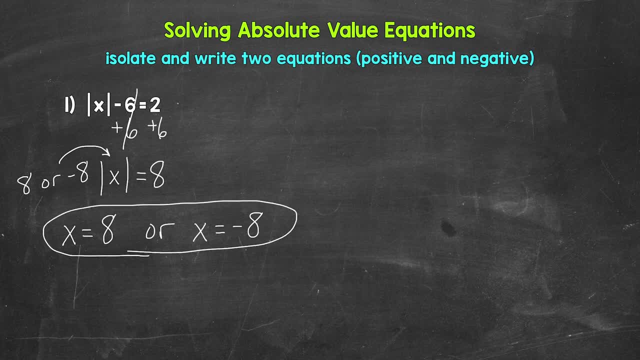 These are our two solutions. Now, in our other examples, we will have to go through additional steps in order to isolate the absolute value of x. So we are going to give us two solutions. We are going to give us one solution: x equals negative 8. Now we know that the absolute value of x equals: 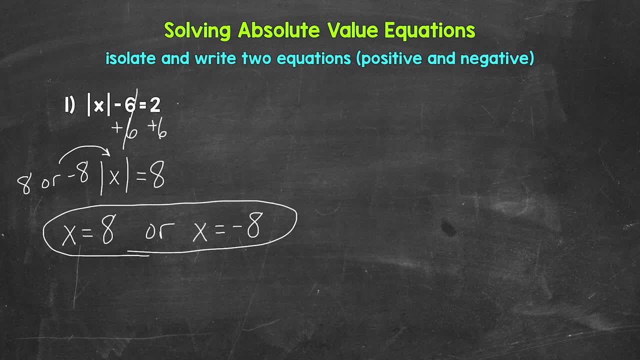 negative 8.. Now we're going toiamente 483.. So we have to isolate the控 Gardens. our solution Now, as we see, we already have twokoa, which is the absolute value of negative 8.. So this in: 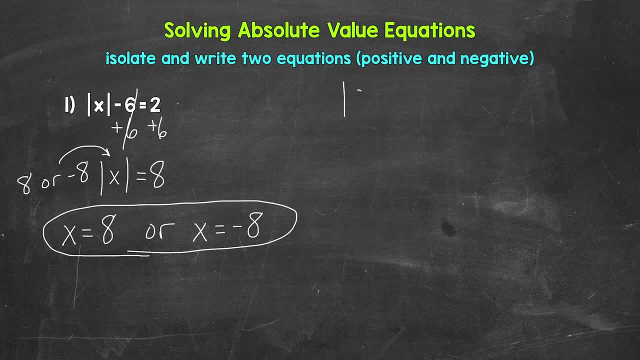 particular seems to be one of the two solutions we are going to have to eliminate the variable. So you'll see what that looks like again as we go through our other examples. Now, once we have our solutions, we can check them by plugging them into the original equation. 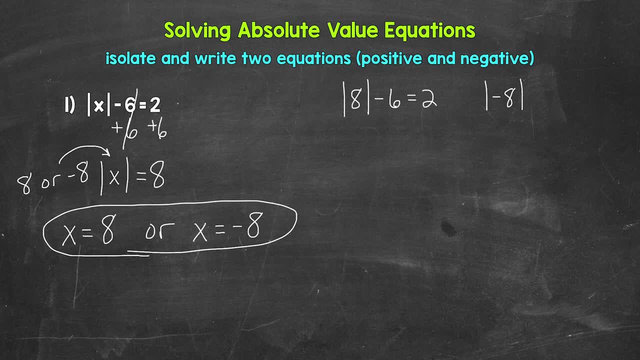 So let's come to the side here. So we have x equals 8, so plug in 8 for x. 6 equals 2. so let's start by checking x equals 8. well, the absolute value of 8 is 8, and then we have: 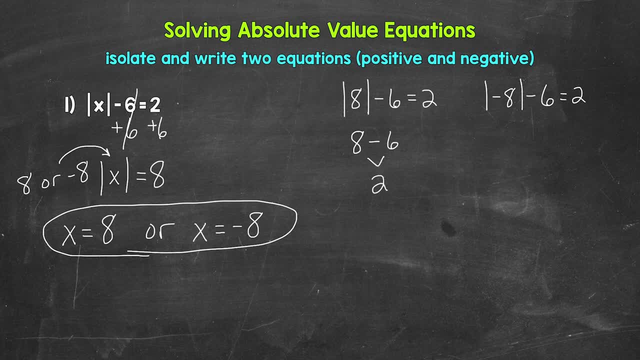 8 minus 6, that does give us 2, so we are correct. there x equals 8. as far as x equals negative 8, the absolute value of negative 8 is 8. so we have 8 minus 6, which again equals 2, so we are correct. 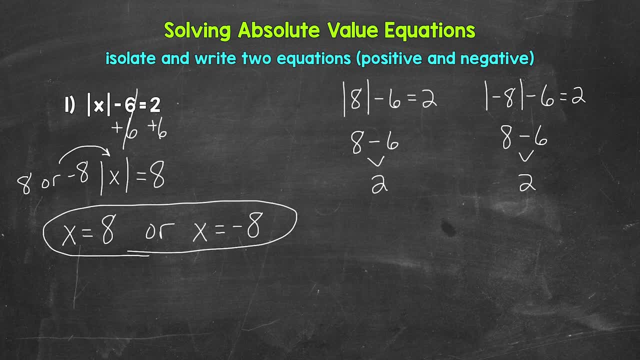 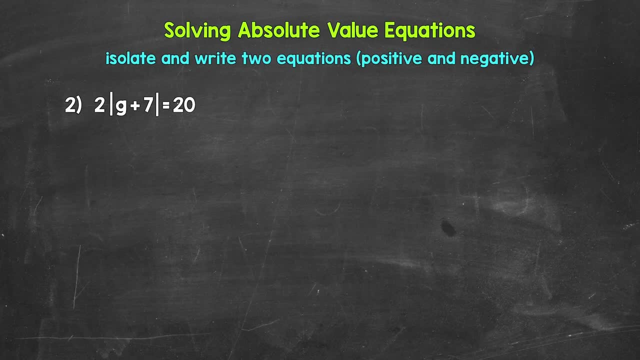 there as well. x equals negative 8. so our two solutions: 8 and negative 8. let's move on to number 2. for number 2 we have 2 times the absolute value of g plus 7 equals 20. is the absolute value isolated? no, so we need to start there now. i do want to mention we cannot use the distributive. 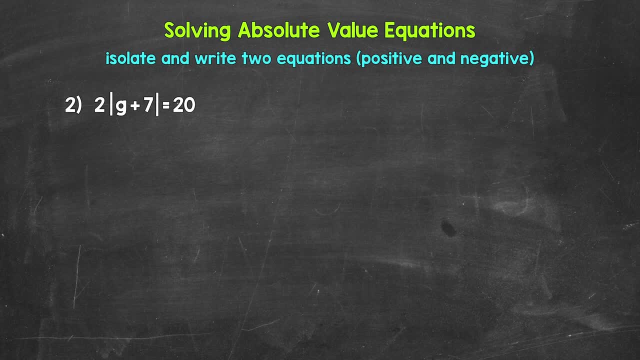 property here with absolute value. those are not the same as parentheses. so just something to keep in mind again: we cannot distribute when it comes to absolute value. we are multiplying the absolute value by 2. so we need to undo that the inverse operation of multiplication is division. so let's divide the left side by 2. whatever we do to one side of an equation, we must. 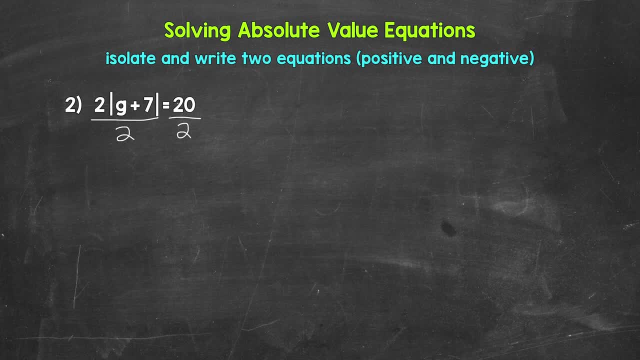 do to the other. so divide the right side by 2 as well. now on the left side, these twos cancel each other out. so we have the absolute value of g plus 7 equals. and then on the right side, 20 divided by 2 gives us 10, so now we have the absolute value of. 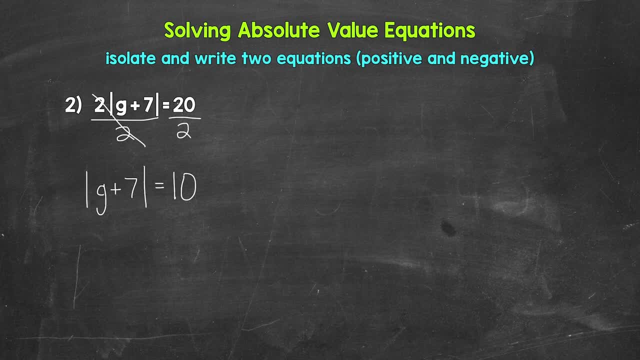 g plus 7 equals 10. the absolute value is now isolated and now that it is isolated, we know that the absolute value of g plus 7 has to equal 10. this gives us two options, two solutions. g plus 7 can either equal 10 or negative 10, because the absolute value of 10 is 10 and the absolute value 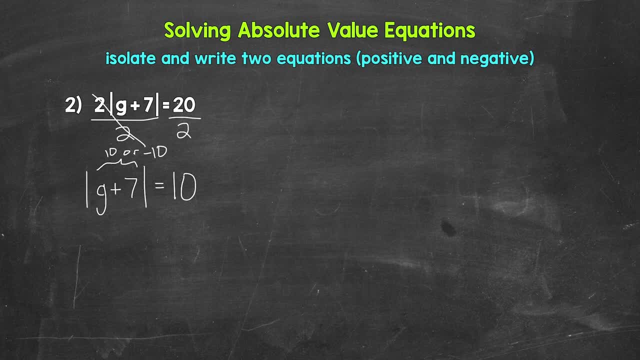 of negative 10 is 10. so we need to write two equations. we have g plus 7 equals 10 or g plus 7 equals negative 10. now we need to solve those to get our solutions. let's start with g plus 7. so let's isolate that variable of g. so we need to subtract 7 from the left side. that means 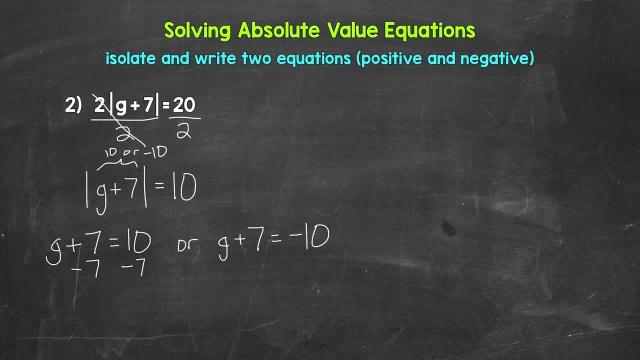 we need to subtract 7 from the right side. these 7s cancel each other out. g is now isolated, so we have g equals. and then on the right side, 10 minus 7 gives us 3, so g equals 3. now let's solve g plus 7. 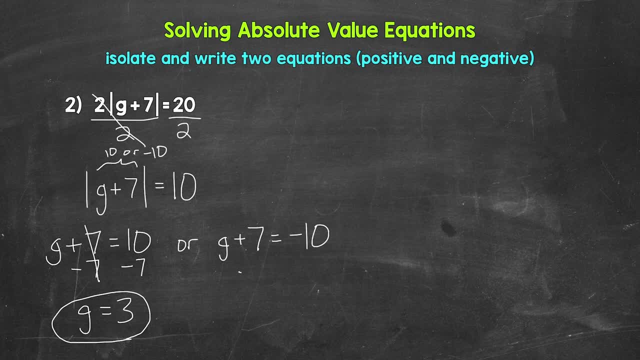 equals negative 10. so let's subtract 7 from the left side and the right side. these 7s cancel each other out. so g is now isolated, g equals. and then on the right side, negative 10 minus 7 gives us negative 17. so g equals negative 17. so those are our two solutions. now let's check those. 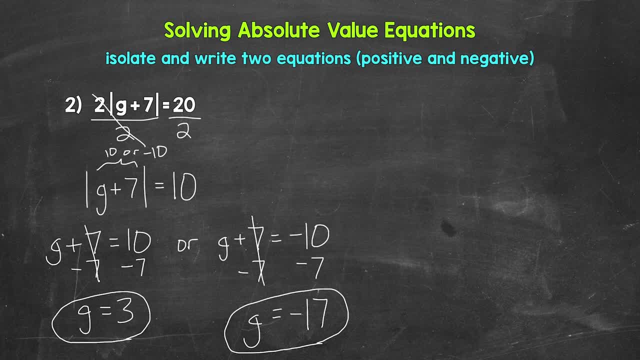 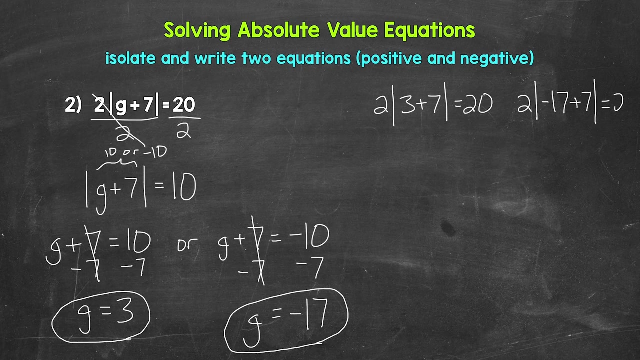 solutions by plugging them in for g and seeing if they work. so we can come to the side here. so we have 2 times the absolute value of 3 plus 7 equals 20, and then 2 times the absolute value negative: 17 plus 7 equals 20. and let's start with 2 times the absolute value of. 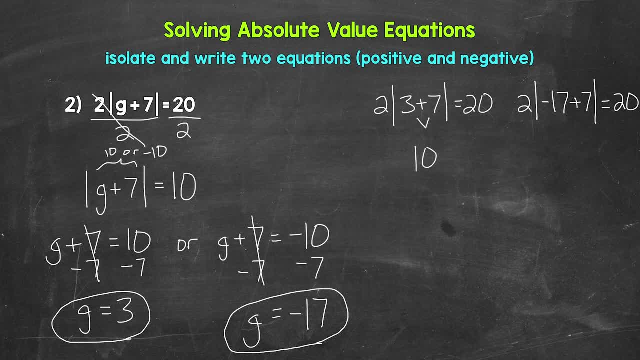 3 plus 7. 3 plus 7 is 10, so we have 2 times the absolute value of 10. the absolute value of 10 is 10, so now we have 2 times 10, which is 20. so we are correct there. g equals 3. let's do 2 times the absolute value of negative 17. 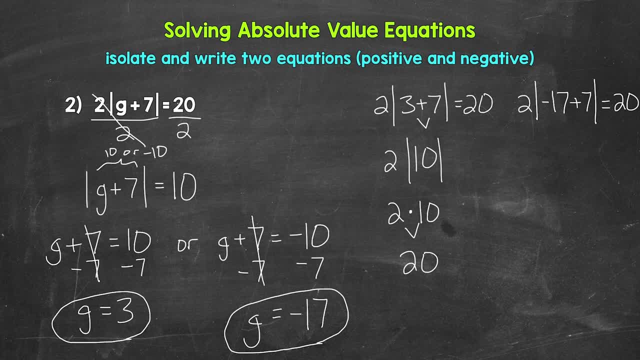 plus 7. now let's start with negative: 17 plus 7. that gives us negative 10. so now we have 2 times the absolute value of negative 10. the absolute value of negative 10 is 10, so now we have 2 times 10. 2 times 10 is 20, so we are. 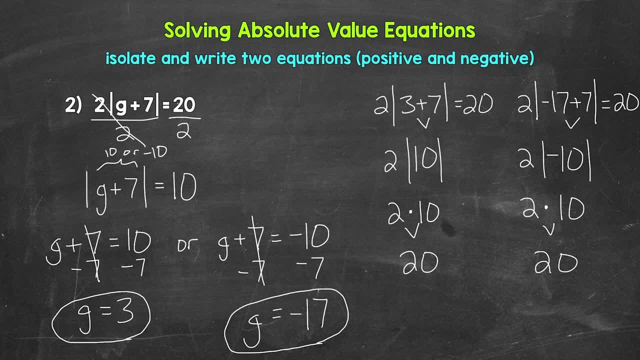 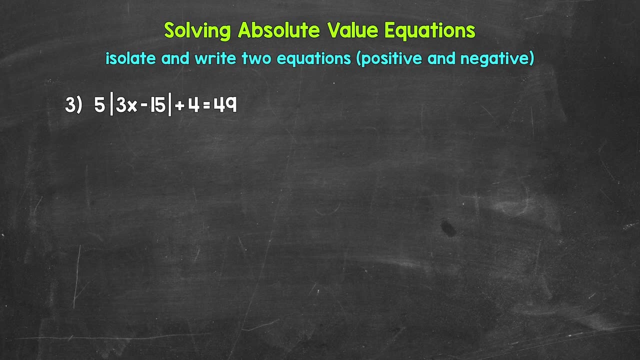 correct there as well: g equals negative 17.. So again, our two solutions here for this example three and negative 17.. Let's move on to number three. Now let's take a look at number three, where we have five times the absolute value of three x. 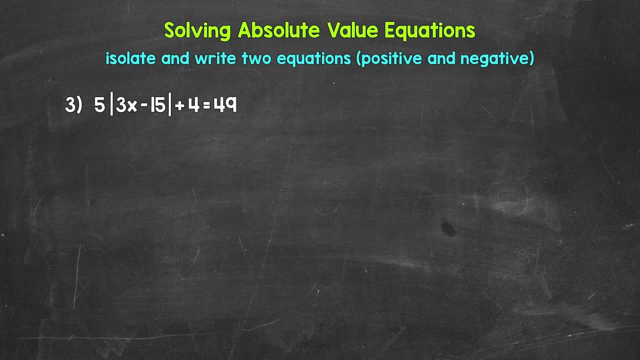 minus 15, then we end: the absolute value plus four equals 49. Now the first thing that we need to do when solving an absolute value equation is to isolate the absolute value. We are multiplying that absolute value by five and then adding four. 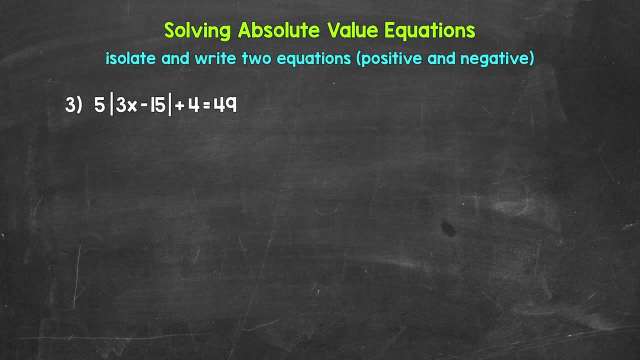 So we need to undo that addition first. The inverse operation of addition is subtraction. so let's subtract four from the left side of the equation. That means we need to subtract four from the right side as well. These fours cancel each other out. 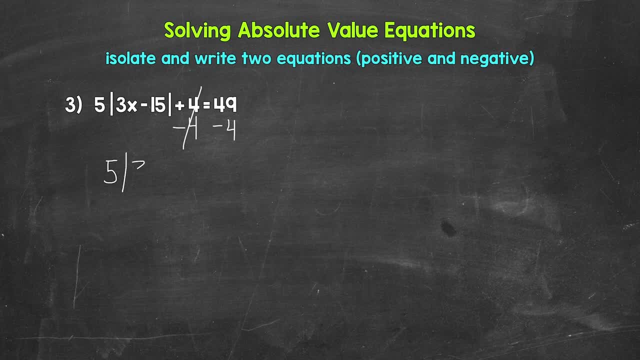 so now we have five times the absolute value of three x minus 15 equals. and then on the right side, 49 minus four gives us 45. And now we have five times the absolute value of three x minus 15 equals 45.. 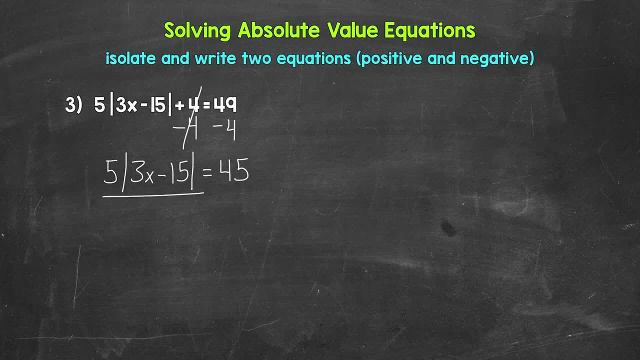 So we need to undo the multiplication. now, The inverse operation of multiplication is division, so we need to divide the left side by five. That means we need to divide the right side by five as well. These fives cancel each other out, and now we have the absolute value of three x minus 15. 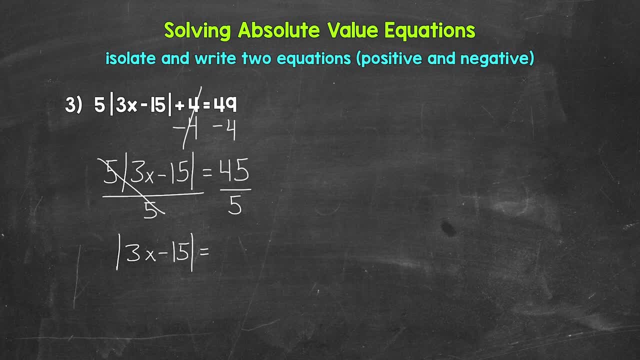 equals. and then on the right side, 45 divided by five gives us nine. So now we have the absolute value of three x minus 15 equals nine. So the absolute value is now isolated. Now we know that the absolute value of three x minus 15. 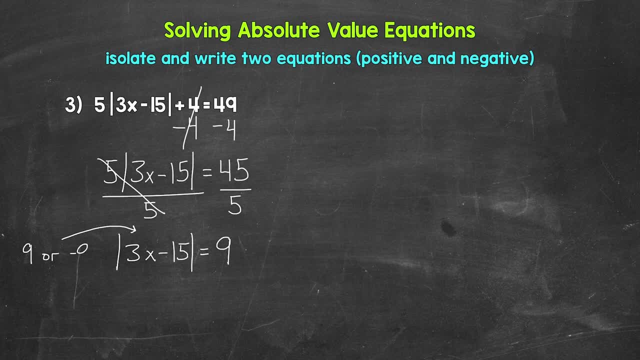 has to equal nine or negative nine. The absolute value of nine equals nine and the absolute value of negative nine equals nine. So we need to write two equations. We have: three x minus 15 equals nine, or three x minus 15 equals negative nine. 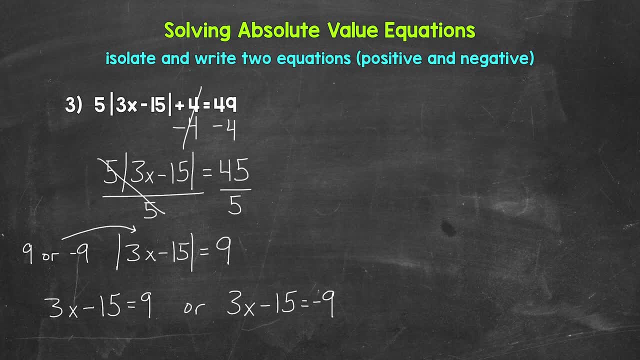 So let's come to the side here where we have more room, and solve these equations. So we have three x minus 15 equals nine, or three x minus 15 equals negative nine. Let's start by solving three x minus 15 equals nine. 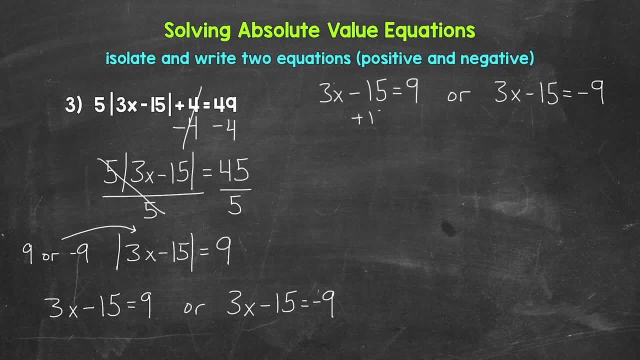 So we need to undo that subtraction. first Let's add 15 to the left side of the equation and then to the right side as well. These 15s cancel each other out, So we have three x equals. And then on the right side. 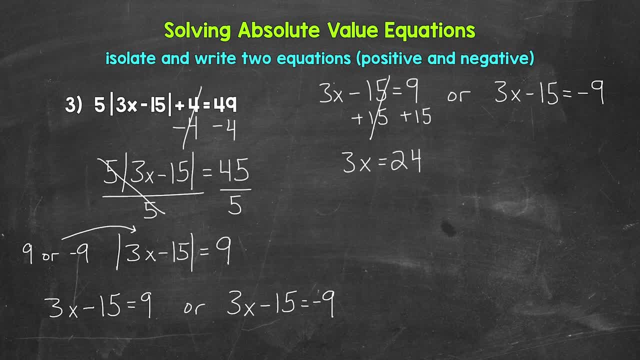 of the equation: nine plus 15 gives us 24.. So we have: three x equals 24, three times x equals 24.. Let's isolate the variable of x by dividing the left side of the equation by three. That means we need to divide the right side. 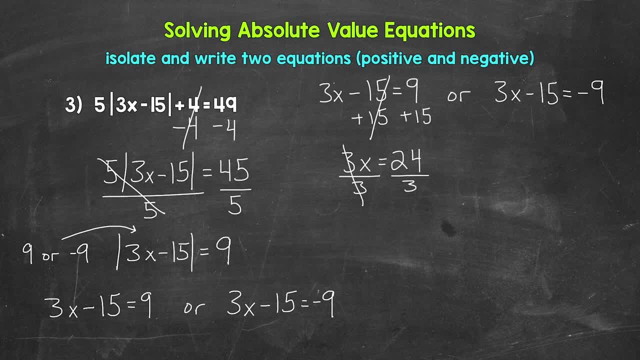 by three as well. These threes cancel each other out. X is now isolated, So we have: X equals. and then on the right side, 24 divided by three gives us eight. So X equals eight As far as three. X minus 15 equals negative nine. 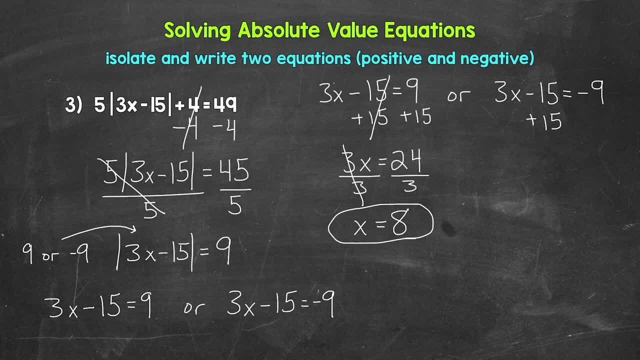 let's undo the subtraction first. So add 15 to the left side of the equation. That means we need to add 15 to the right side as well. These 15s cancel each other out. So we have three X equals and then negative. nine plus 15 gives us a positive six. 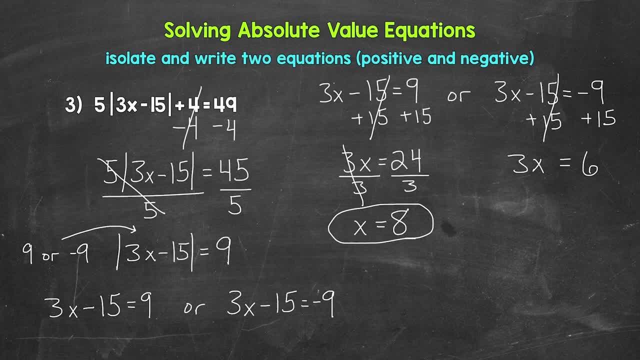 So now we have three. X equals six. Three times X equals six. Let's isolate X by dividing the left side by three. That means we need to divide the right side by three as well. Taking a look at the left side, these threes cancel each other out. 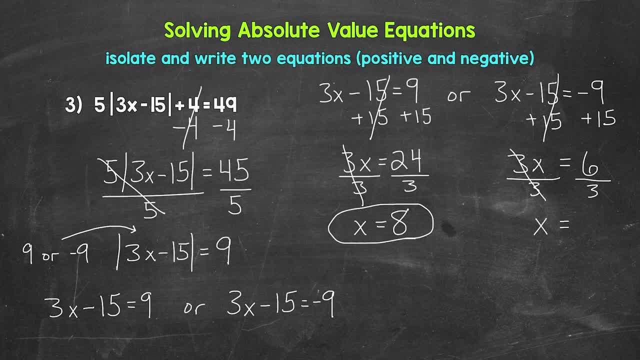 So we have X equals. and then, on the right side of the equation, six divided by three gives us two. So we have X equals two. And those are our two solutions. Now let's check these solutions by plugging them in to the original equation and seeing if they work. 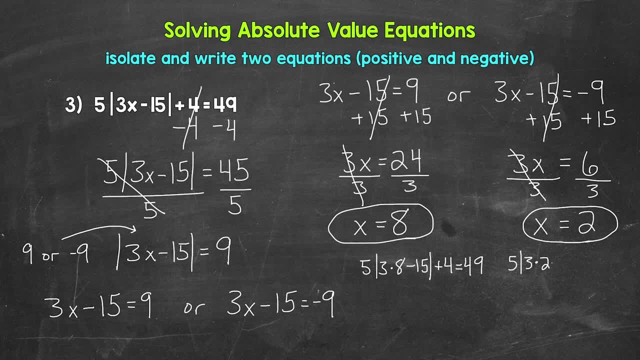 Let's do that. So let's run this again. So let's do this again. Let's start with checking. X equals eight, So within the absolute value, we have three times eight, which is 24 minus 15.. That gives us nine. 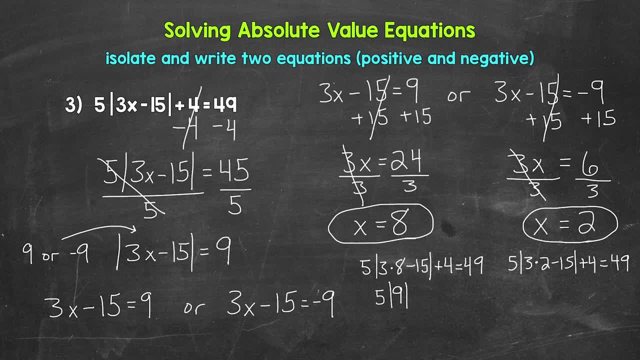 So we have the absolute value of nine. now, five times the absolute value of nine plus four, The absolute value of nine is nine. So we have 5 times 9 plus 4.. 5 times 9 plus 4 is 49, so we are correct there.